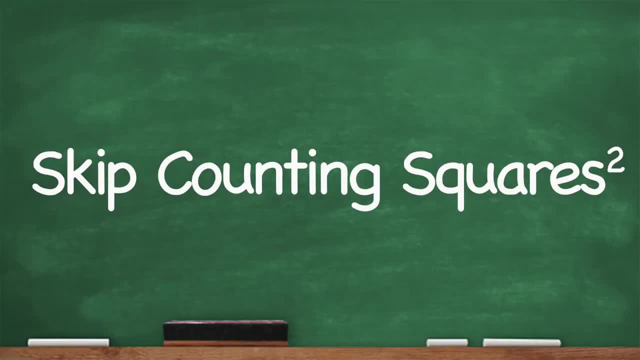 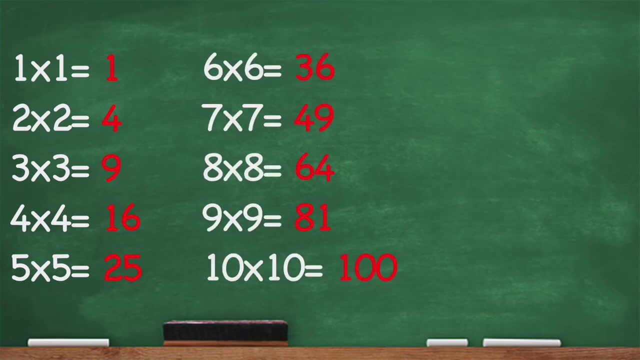 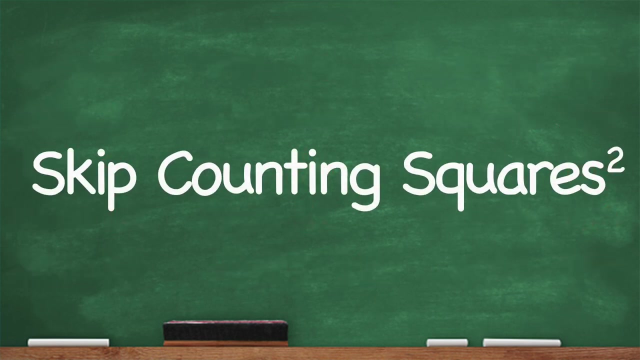 Week 10. Skip Counting the Squares. Week 11. Skip Counting the Squares. 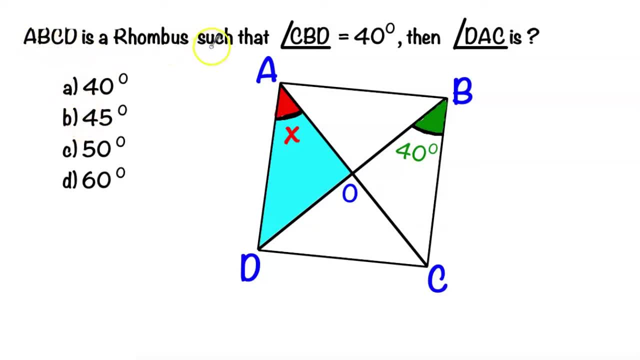 Hi, all it's SuperEasyMath. Given that ABCD is a rhombus such that CBD is 40 degree, we need to find angle DAC. Is it 40, 45, 50 or 60?? Pause the video if you want to give it a try, And now let's go ahead into solution. 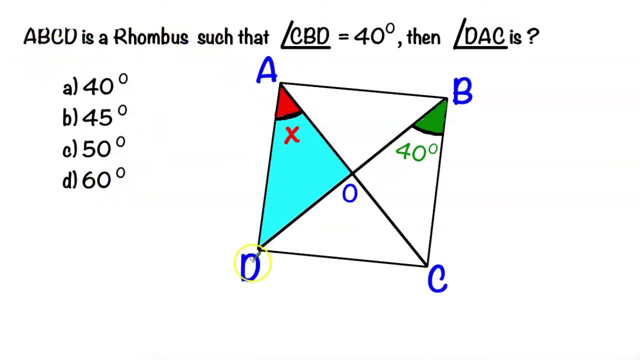 Since ABCD is a rhombus, then opposite sides are parallel. In this case AD is parallel to BC. So here we have two parallel lines and another line intersects this parallel line. The angles that form a letter Z is called alternating angle. So this angle is equal to this angle and these angles are equal. Another alternating angles here: this angle and this angle. 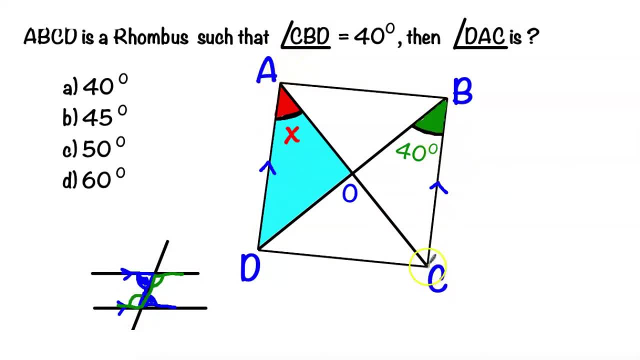